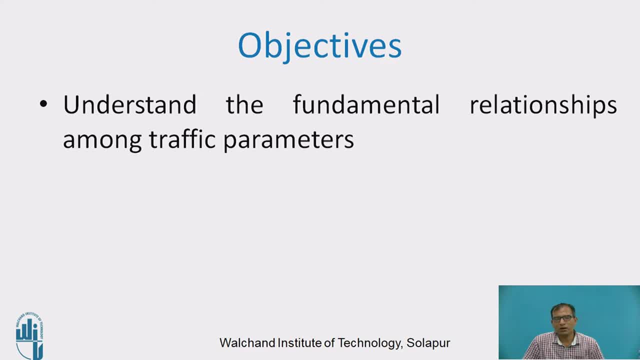 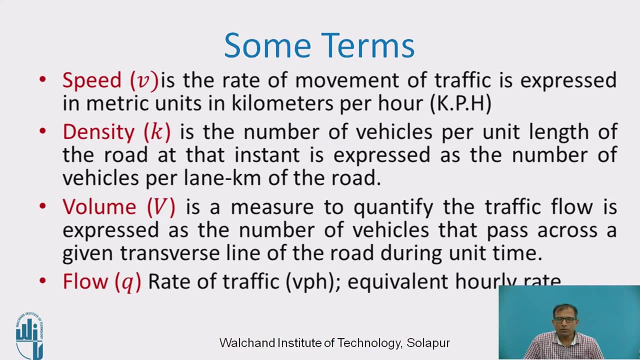 At the end of the session, students will be able to understand the fundamental relationship of the various traffic parameters. Before we go for fundamental relationship, let us understand some of the terminologies related to the traffic characteristics. The speed is one. speed is the rate of movement of traffic. It is expressed in Kmph and density. 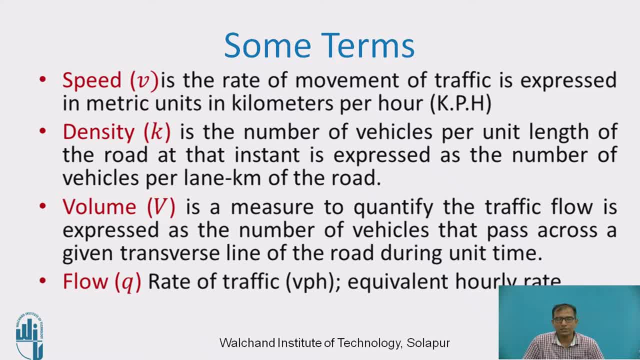 is number of the vehicles per unit length of the road at that instant and it is expressed in number of vehicles per kilometer of the road and volume. we know that it is the number of the vehicles per kilometer of the road And the speed is one. speed is the rate of. 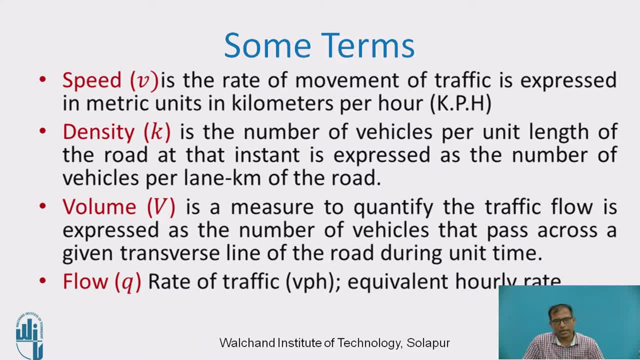 vehicles flowing on a transverse line per unit time. Usually we take 15 minute is the unit time and to convert this 15 minute volume into hourly rate of flow- that is what we call as a flow, that is, rate of traffic equivalent to hourly rate- We can convert this 15 minute. 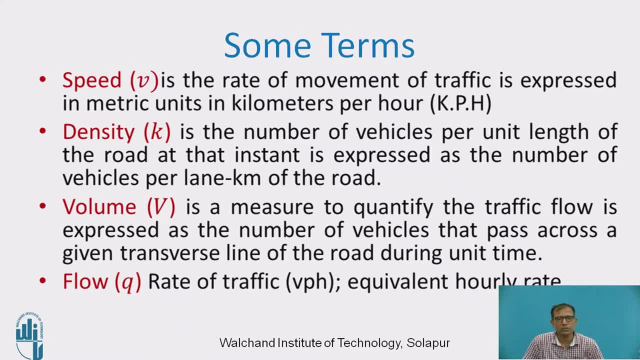 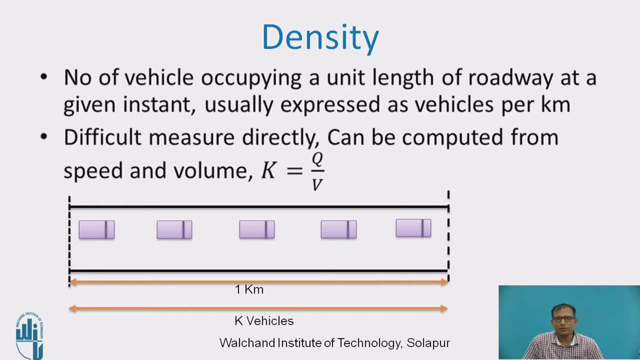 volume traffic into hourly rate of flow. So there is no difference between the volume and flow. only then we flow is expressed in hourly rate. Now what is the density? Density is number of vehicles occupying a unit length of roadway at a given instant. So usually it is expressed in vehicles per kilometer. If you say the 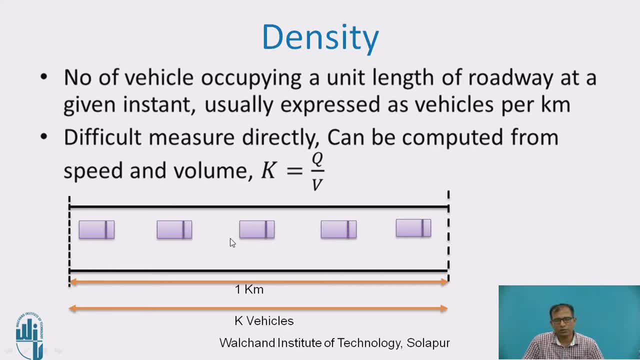 in one kilometer length. how many number of the vehicles are spaced in one kilometer length? So that is, K is indicated by the density In sight. it is very difficult to measure the K value, which is we know that we have to get elevated observation. 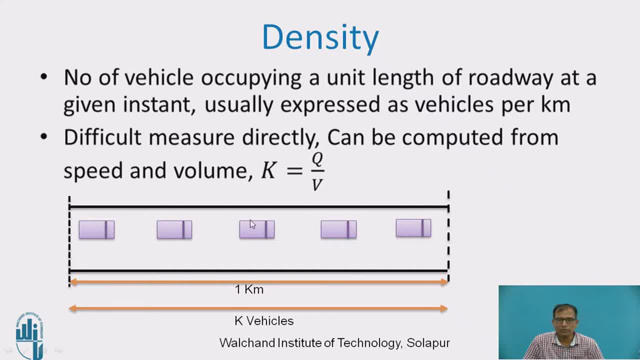 So that one kilometer length is purely visible from that elevated observation, So that we can count the number of the vehicles are spaced in one kilometer, or whatever the distance given to you. So, with the relations of this flow, Q is what the flow and V is your speed. 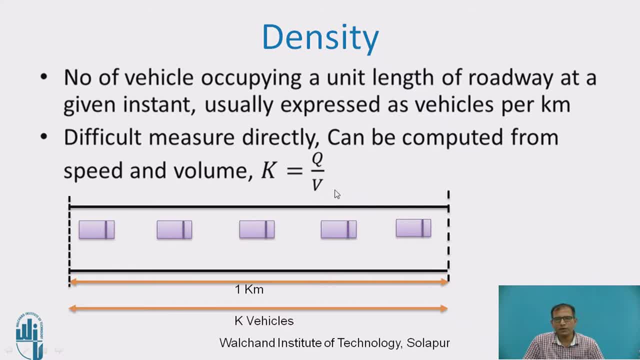 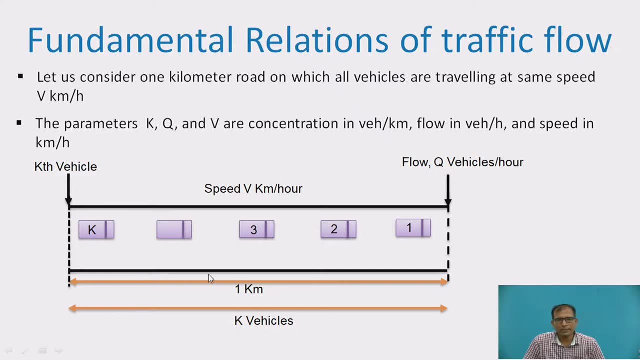 So, having this the flow value and speed value, we can able to determine the. what is the density in number of vehicles per kilometer? So that is K equal to Q by V, So the fundamental relationship of traffic flow. So this is the one kilometer length over here on which the all vehicles are travelling. 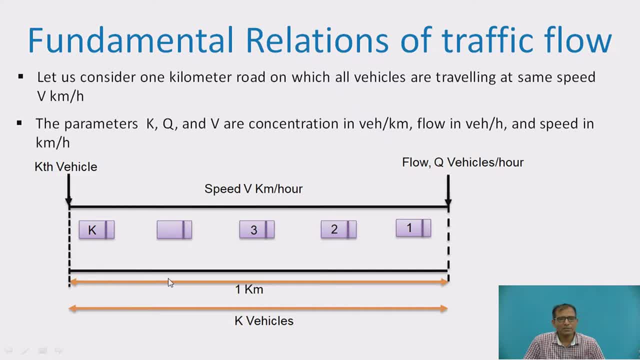 at a same speed, V kilometer per hour, And the parameters the density, K and Q flow and V speed are. the unit is vehicle per kilometer, flow in vehicles per hour and speed in kilometer per hour. So let us try to understand the relationship between the K, Q and V By definition. 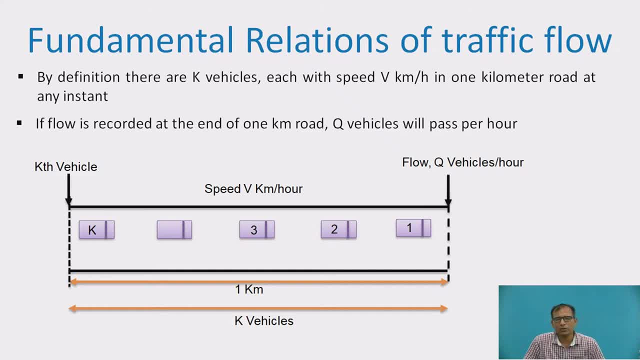 there is a K vehicles, each vehicle with a speed of V kilometer per hour in one kilometer road. If you take the Transverse line versusadı a unit time of for a flow, it is taken as 1 hour time. So in this one Kth vehvern is the density vehicle and these are the number of vehicles. 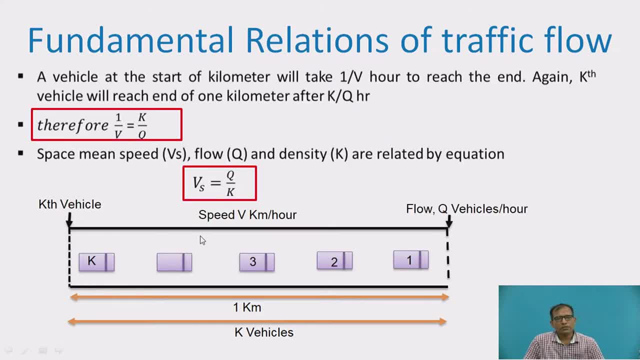 up to the Kth vehicle. So a vehicle at the start up the one kilometer will take 1 by V hours. That is a time to turn a 1 by V hours into one hour time, But the velocity of a, that is the time to complete this. the unit distance of 1 kilometer, it is 1 by V hour. 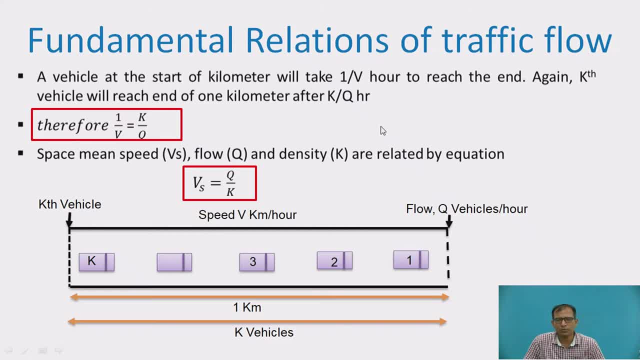 That is the relationship we are using. that is, speed equal to distance upon time and time equal to distance upon the speed. So again, the kth vehicle will reach at the end of this 1 kilometer after the k by q hours. So we can take that. the vehicle will take 1 by V. 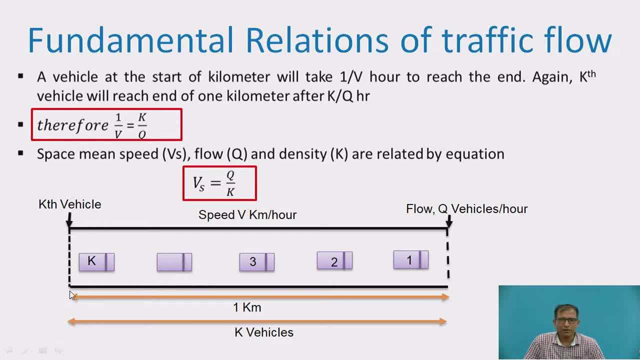 k hour to reach the this end are the kth vehicle. This kth vehicle will reach the end of 1 kilometer after k by q hours. So equate this 1 by V to k by q, So that will get the relationship. 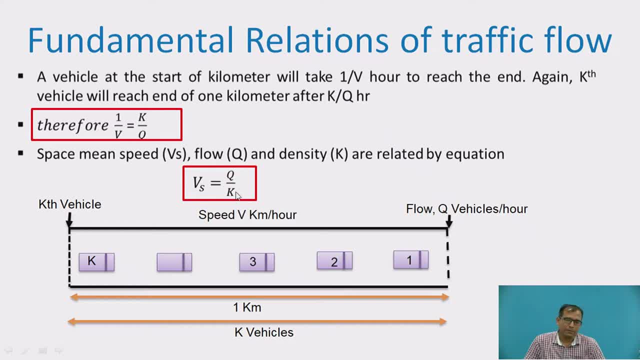 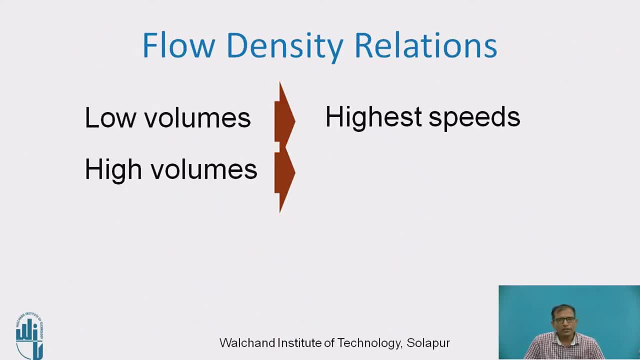 that is V S equal to q upon k. That is, q is what the rate of flow and k is our density. Now we know that the as the relationship between these parameters Low, low, low volumes, highest speeds. So as the speed increases, the volume is get decreases. This is already. 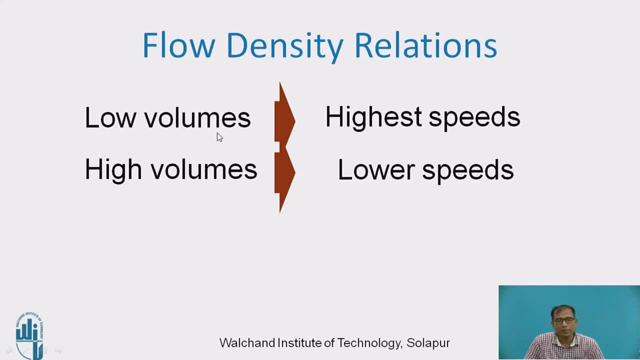 we know that this is because of the gap between the each vehicle. So as the gap between the each vehicle get increases due to the highest speed, the volume will get decreases And in the lower speeds we get high volume. but is rather, you say that lower speed, we say if? 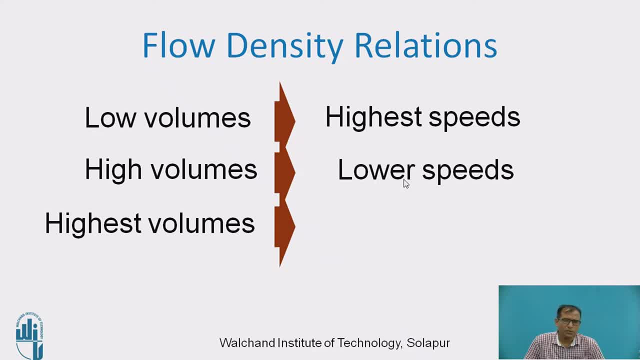 we say that it is optimum speed. So at optimum speed or optimum headway distance we get the higher volume. And highest volume is also obtained at density. optimum density And the maximum density is possible when we have the speed is very low. So it means the gap between 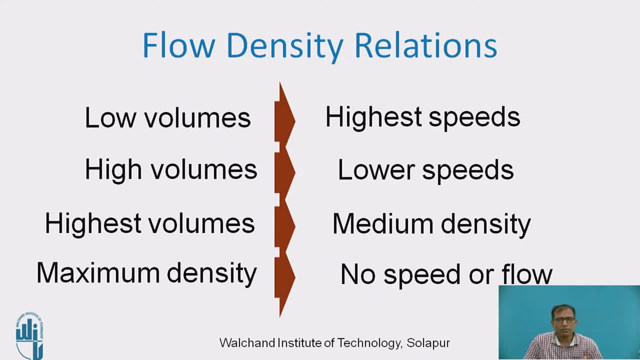 the each vehicle, that is, distance from front of the vehicle to the front of the vehicle. that distance is less due to the speed is low and that case you may go for maximum density. That is the relationship we are using. just now. we have derived the equation. 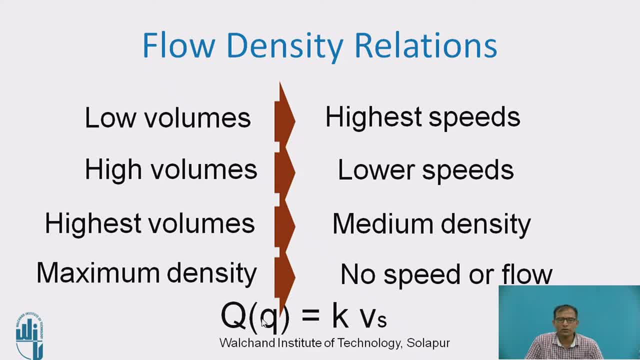 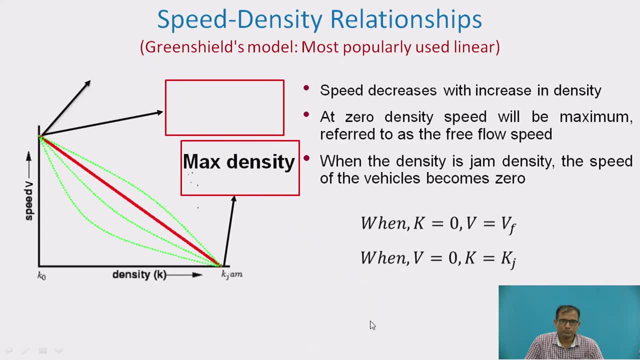 That is q equal to k into v s. So if you want to find out the q value, you can. you required the density and the this speed value. Now here we will try to understand the speed density relationship. you can see that as the density increases, the speed will get reduces. This 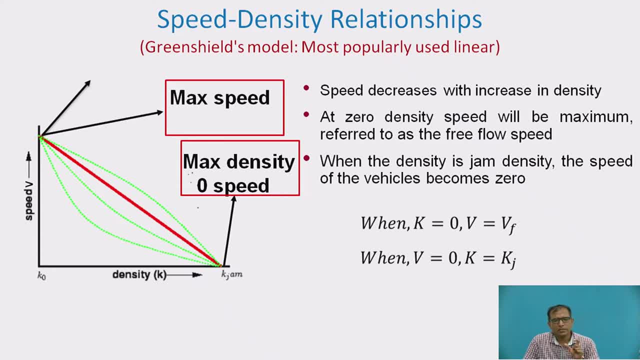 is reason. the reason because the distance between the each vehicle get reduces as the speed reduces. Due to that, the density will attain maximum speed. So this is the reason for the maximum value. So at free speed you can see that the density is 0 because the 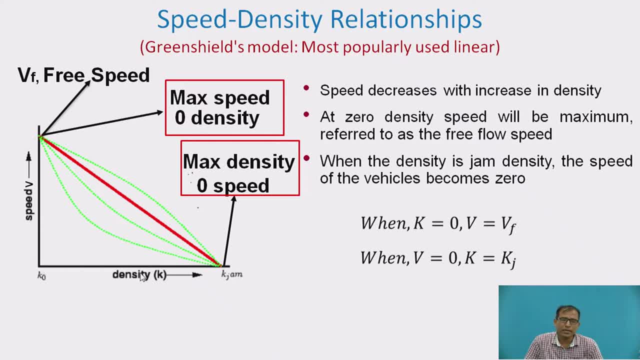 at high speed or the free speed, you get that the spacing between the vehicle is very high And due to that you will going to get the 0 density at a speed of v f free speed, And as the density increases the speed will get decreases. So when k equal to 0, your v will. 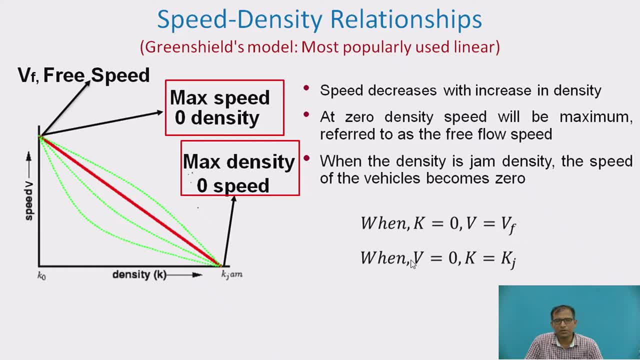 become v f, So the speed will become to free mean speed. and when v equal to 0, your k equal to k j, So k j is nothing but your jump density over here. So that is when speed is 0 you will. 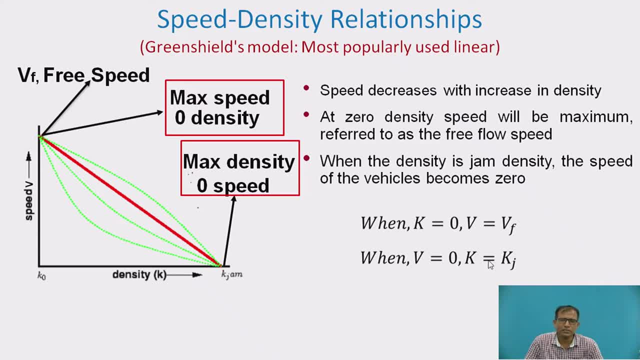 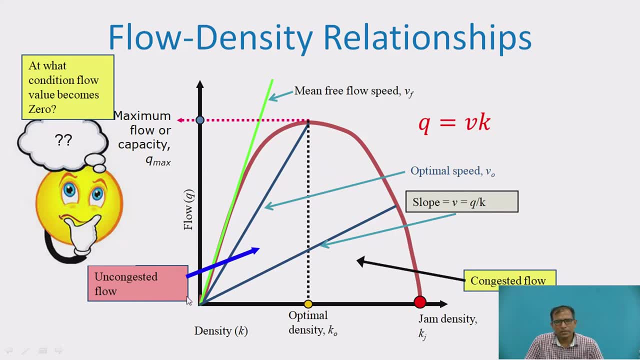 see that all the vehicles are in congestion condition or it is in stand still condition. So another, the relation between the flow density relationship. you can see that on the y axis we got flow rate of flow in hour and this is the density way. number of vehicles. 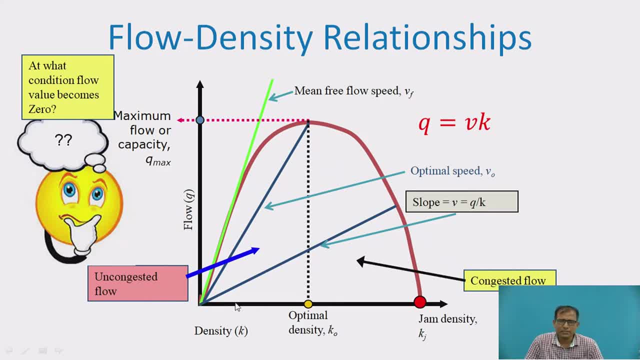 per kilometer. So when the velocity increases, you can see that the up to a certain point you can take half of this, the curve. on this side you can see that it is a stable flow or uncongested flow, because as the flow is increasing means your speed is also increasing. So when speed 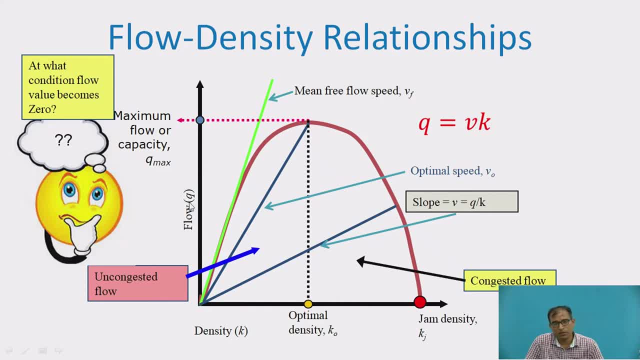 is increasing. up to a certain point, the flow is maximum. Beyond this point, beyond this point, even flow is also get decreases. after the, beyond the speed- that is very high speed- the flow is also get decreases. So if the as the speed decreases, you see that the flow also starts decreasing. on this, 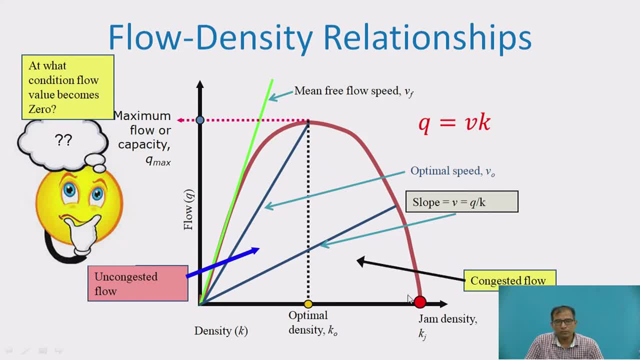 line And at certain point, when flow becomes 0, it means the gap between the each vehicle is very, very small and speed is lesser. at that point the jump density will happen. So it means long queue length will happen or congestion flow happen at this jump density. 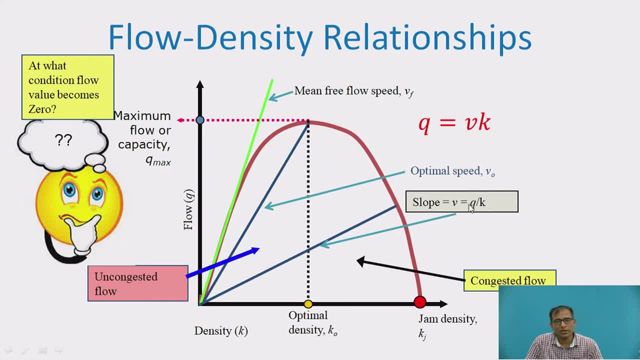 The slope of this line. it gives the speed, or we can say that we have in the. You see the slope of this line, that is q by k. that gives the your speed, optimal speed. Now you can pause over here and think for a moment at what condition the flow value. 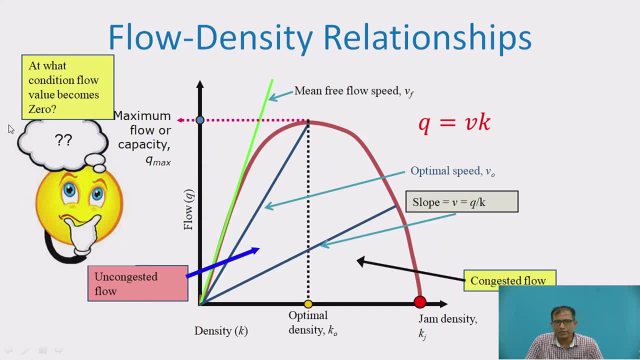 becomes 0.. You can think for a moment and answer this question: when will be the flow will become 0 or at what condition flow will becomes 0.. So I hope you will. I hope you are going to get the answer for this question. the flow becomes 0 when the density is 0 over. 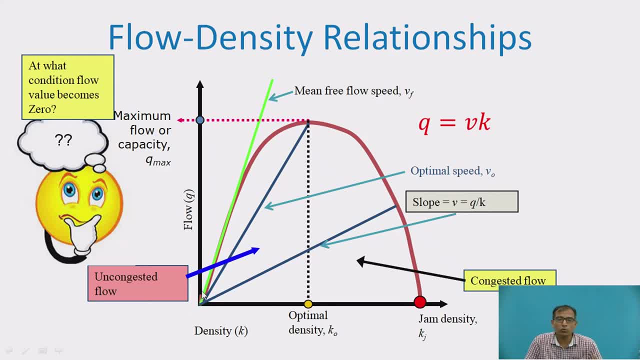 here. So when the 0 density is there, it means there is no vehicles is there in that particular stage. that possible condition is the possible or vehicles are going with very excessively very high speed. It means the you cannot measure the speed of the vehicle. that condition, the 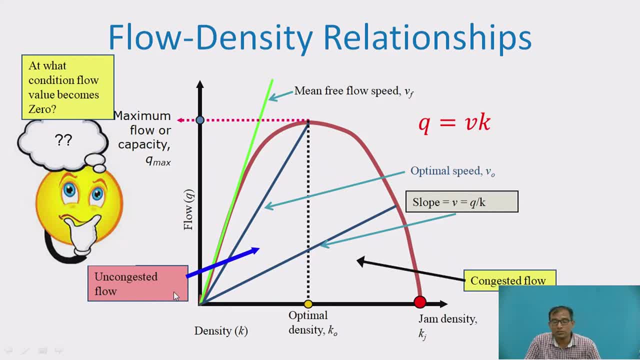 headway distance is very, very larger and that condition, even flow, is also 0.. So when density is 0. Your flow is also 0 because there is no vehicle exist in that stretch. due to that, flow is 0.. Another way: when there is your speed, vehicle speed is going very excessively high. that 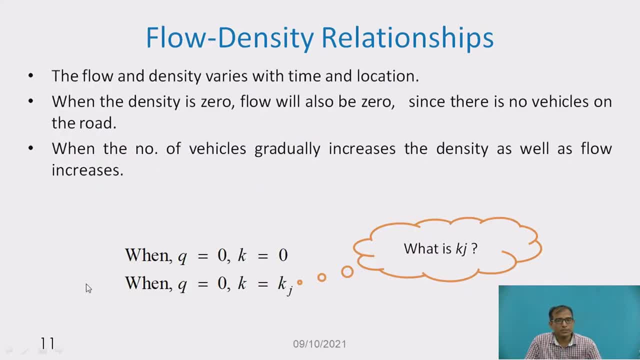 condition also, your flow will also be 0. So that is the reason: the when q equal to 0, your k is also 0. that is, when flow is 0, your density is 0. In this condition you can see that there is no vehicle is exist in this condition in that particular stretch. that is the reason. 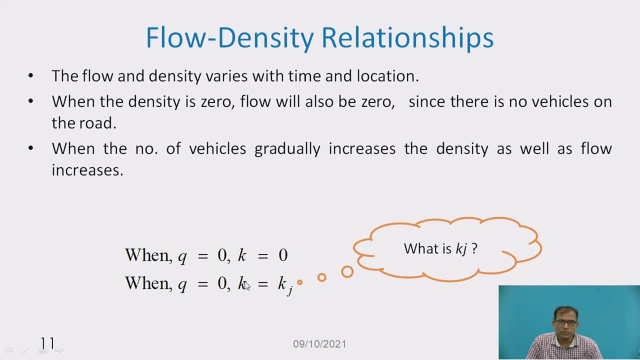 you see that The density is also 0. So when flow is 0, it means the when certain, when speed reduces, the flow also get reduced and this condition happens for way that vehicle is not at all moving in that particular stage, that condition, the density will become the jump density. 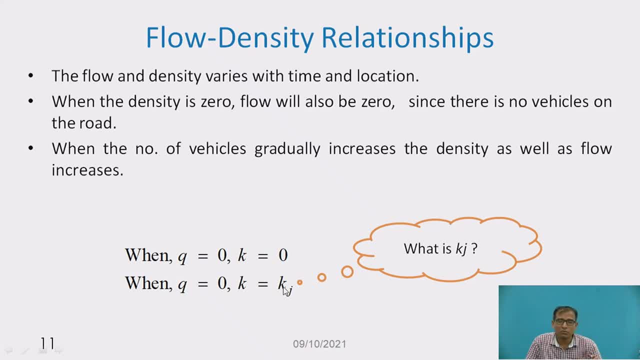 This is jump density, where all vehicles are standstill and going with very crawling speed in that particular stream. So that is reason to the vehicles are not at all moving or you are not getting any flow value with that standstill condition. The standstill condition is nothing. 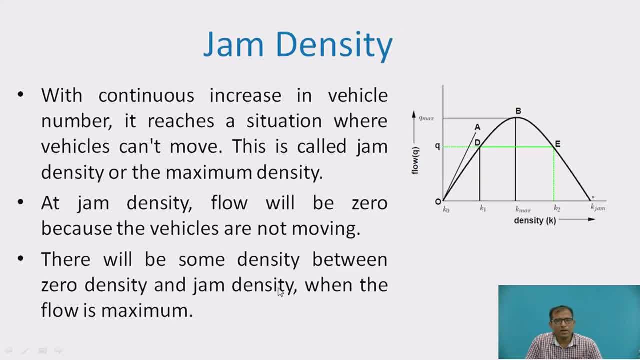 but your k j value. So jump density. this is the relationship of the flow and the density. So that is already. we have seen that as the density increases, your flow is going to be, up to certain point, the at optimum density. this point is called as the k max at optimum. 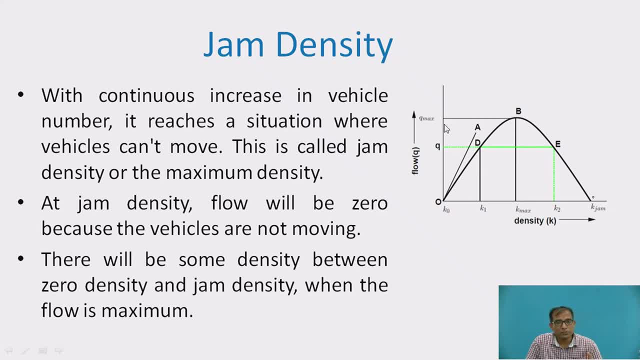 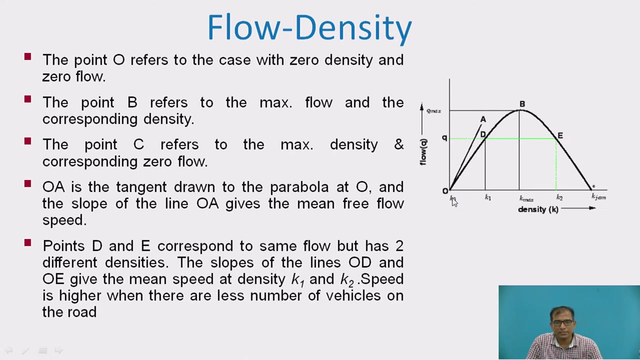 density. you see that optimum flow, that is optimum speed, optimum flow, optimum headway and optimum your the speed, In that condition the flow is maximum. and after that, as the density increases beyond this optimum point, you see that flow starts reducing. So this is the flow and the density relationship, this already we have discussed. So here the 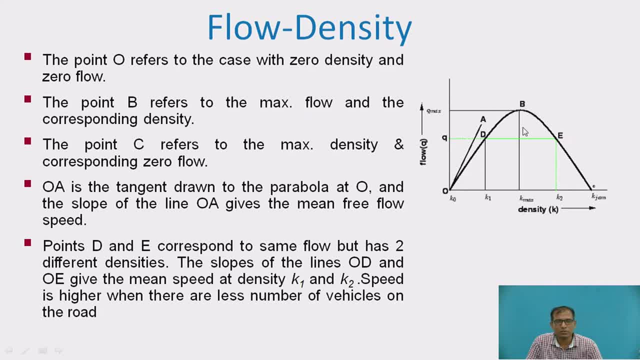 point b refers to the maximum flow. So this point b refers to the maximum flow And point c refers to this is the point c refers to the maximum density, or this is also called as a 0 flow or a jump density. this point is a, c and o. a is the tangent over here. 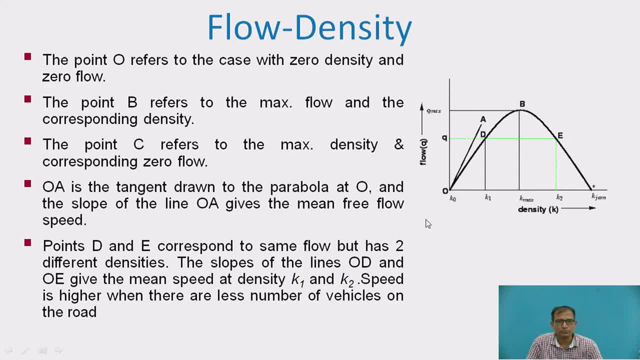 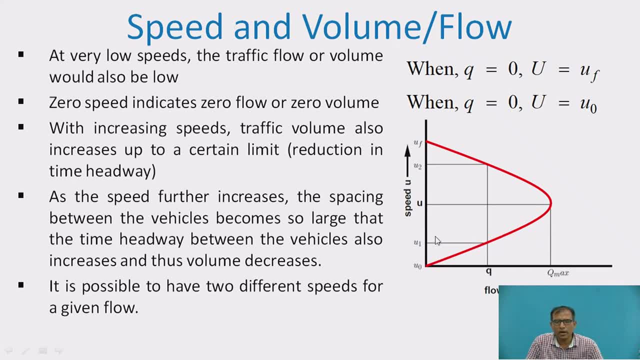 and slope of this. you can get the, your speed value, Then the speed and volume relationship. in this x axis we have got the flow value and y axis we have got the speed in k, m, p, h. When q equal to 0, that is the when the flow is. 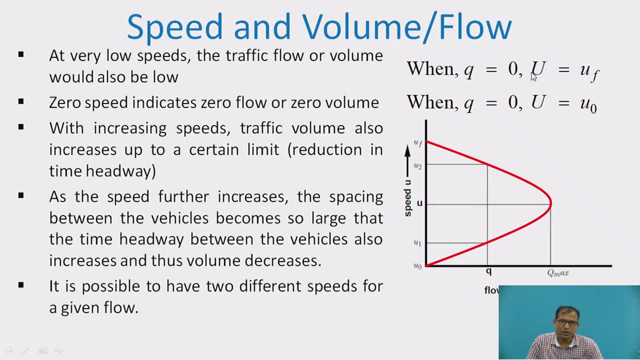 0. Your speed is also 0. So here the u equal to u f. So when flow is 0 means the it is going to get maximum speed, As I told you. when flow is 0, it means you cannot measure. 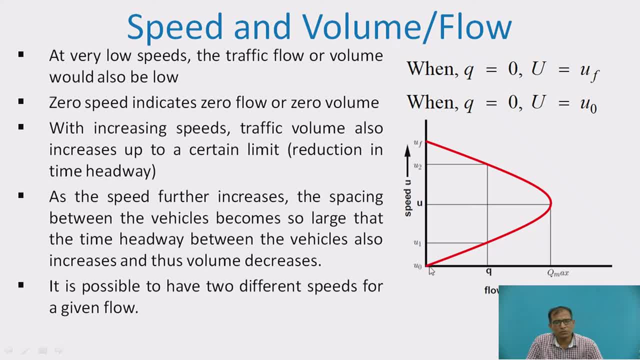 the vehicle speed at all. So this is possible. condition: flow is 0. in this condition means vehicles are going with very this free mean speed. So that is the reason. and when q equal to 0, u equal to u naught. So here the 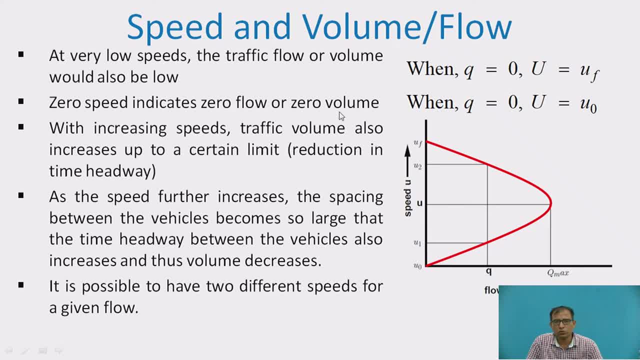 This is the condition. 0 speed indicates the 0 flow or 0 volume. with increasing speed traffic volume also increases up to a certain limit reduction in the time. it We can see that up to this optimum speed your flow will be maximum. So after this point the speed reduces.